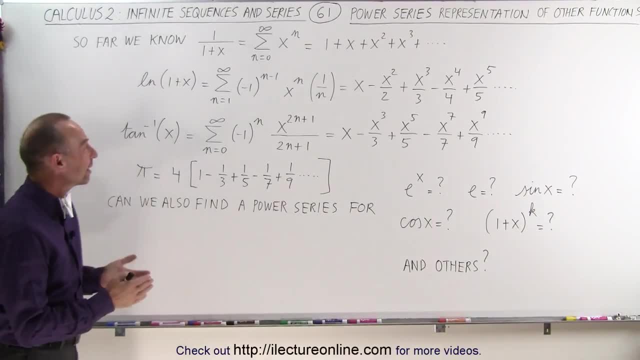 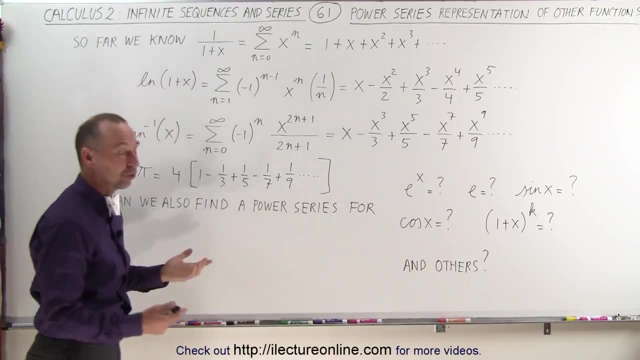 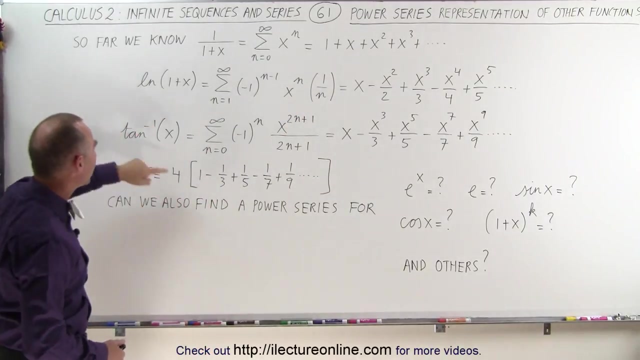 Welcome to ElectronLine. So far, we've been able to take some of these key functions, such as 1 over 1 plus x, and turn them into an infinite power series like that This is also known as a geometric series. We've taken the natural log of 1 plus x and written it as a power series. We've taken the 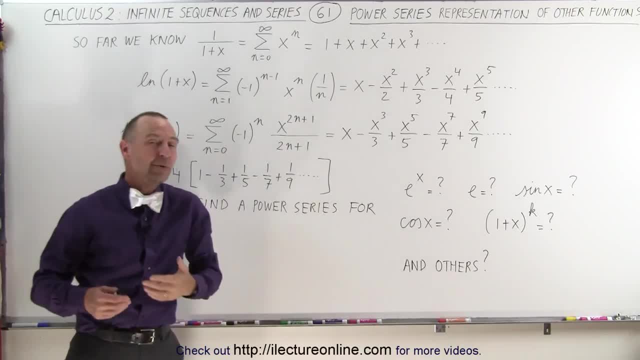 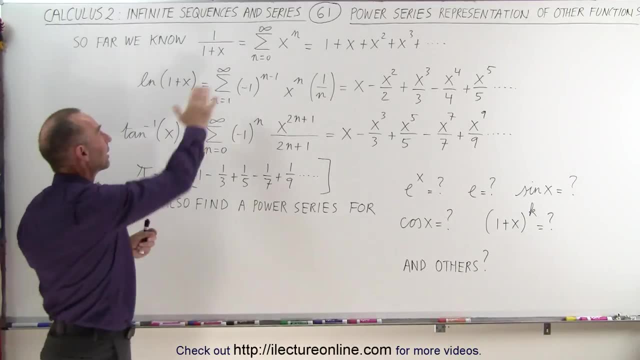 arctangent of x and written it as a power series, And then we've used other techniques, such as taking this as the initial step and then taking other functions and making them look like that to be able to write out an infinite series for those. We've also used techniques such as 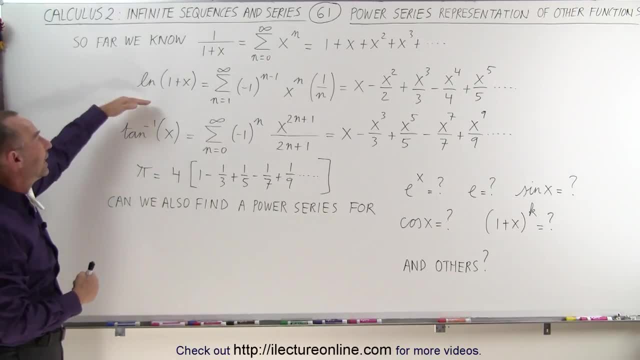 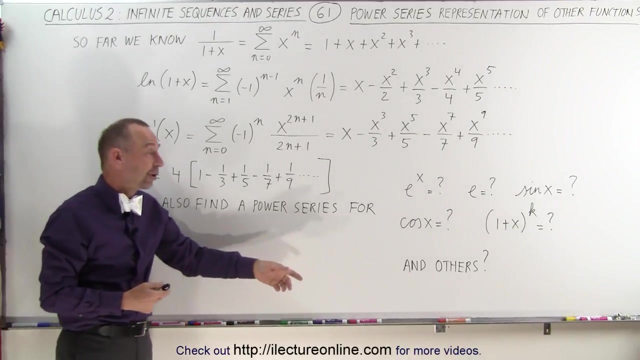 differentiation or integration, to come up with infinite series or power series for other functions related to these and even not so related to these. We've even been able to find the number pi using the power series. Now the question is: can we also find a power series for other very famous functions? 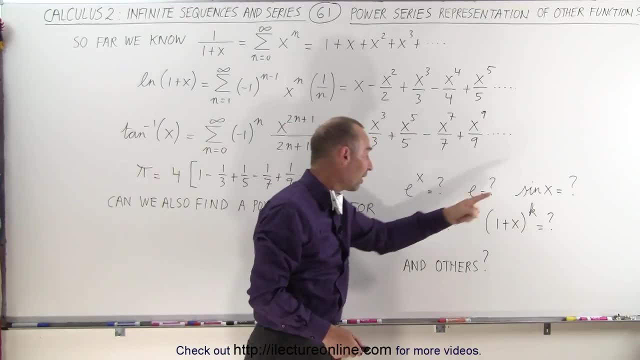 such as e to the x, Maybe for the number e, The sine of x, The cosine of x? How about the binomial of x? How about the cosine of x? How about the binomial of x? How about the cosine of x? How about the binomial? 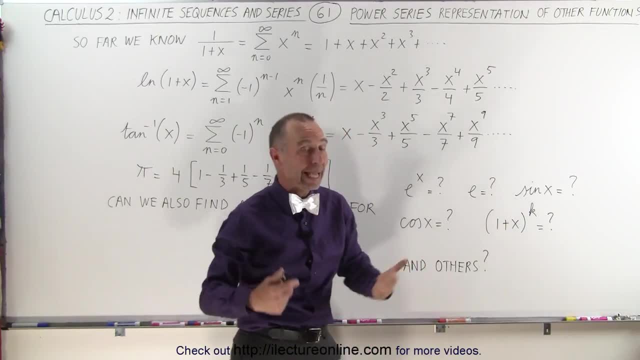 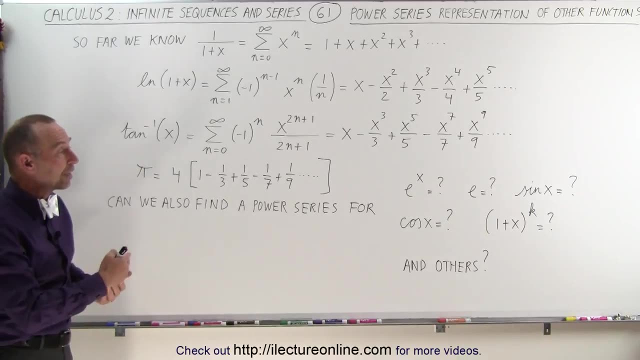 of the expansion of 1 plus x raised to the k power, where k can be any integer and maybe even others. and the answer, of course, is yes, and that's what we intend to do: show you how to find the power series, or infinite series, for many of these other functions, and it's amazing what you're able to do. 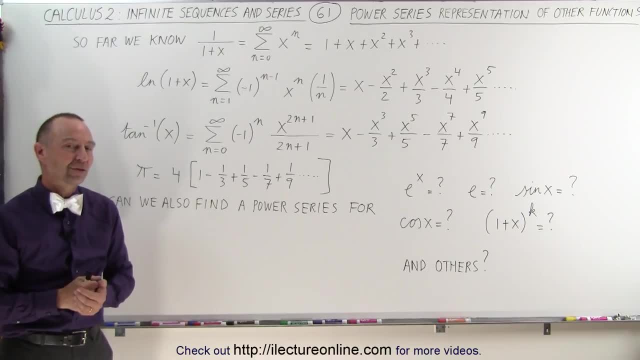 once you're able to write these as those power series functions or those power series forms of the particular functions. So if you wonder what we're going to do next, we're going to tackle some of those challenges as well. That's how we do that.